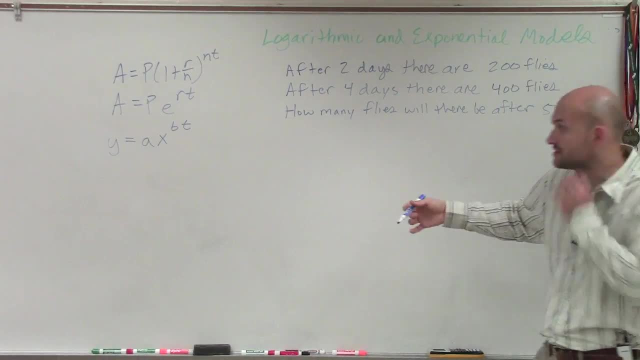 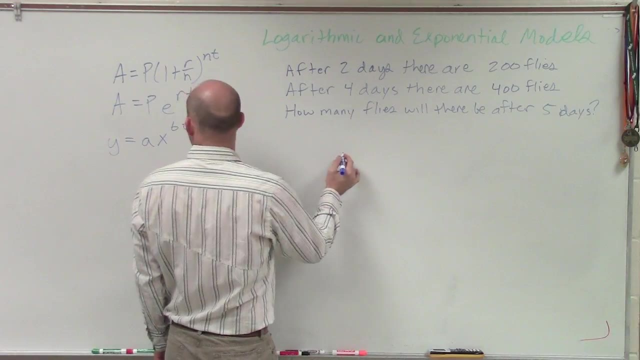 We know what the time is, though, and we know what our final value is, So what I'm going to do is I'm going to use this model to represent two different equations we have here. So if I was going to use this model here, 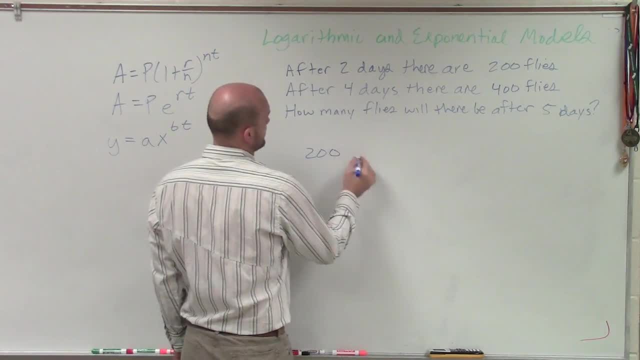 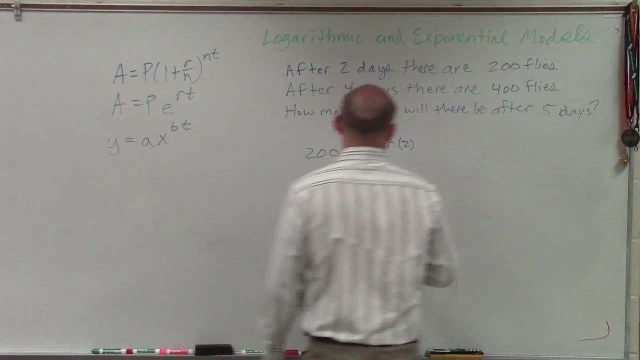 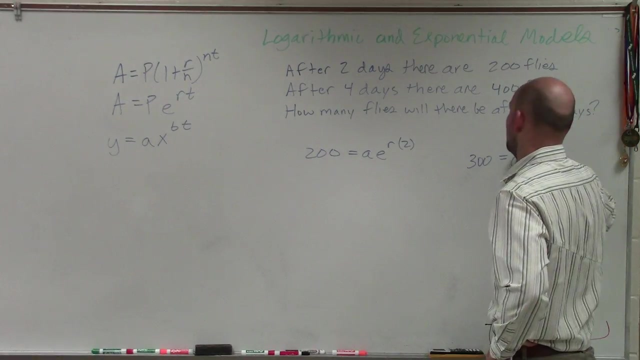 y equals a times x to the b to the t. I can say that 200 equals a times e raised to the r times 2.. And I could also say that 300 equals a to the e- I'm sorry- a times e raised to my r times 5.. 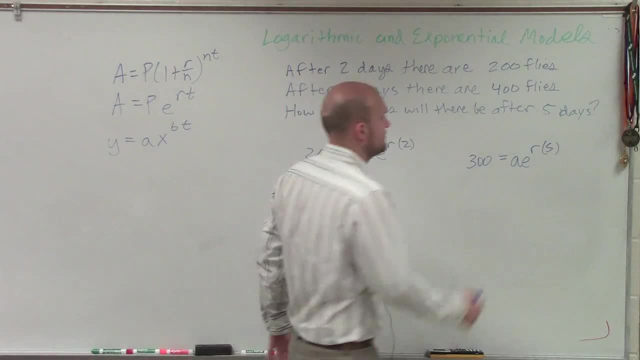 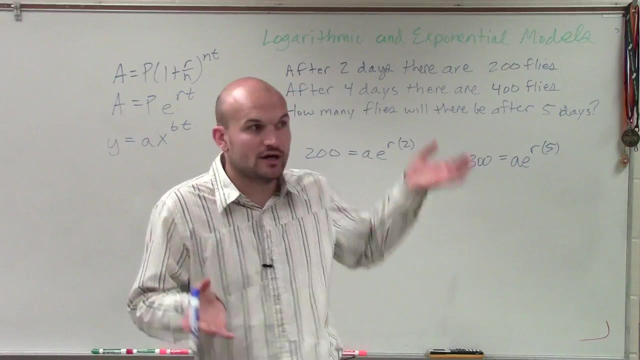 Now, in this case, ladies and gentlemen, we don't know. That's a 5.. In this case, we don't know what the initial amount is after one day, right? All we know is after two days, there was 200 flies. 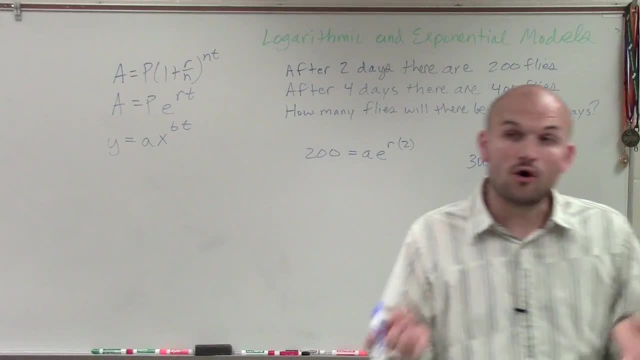 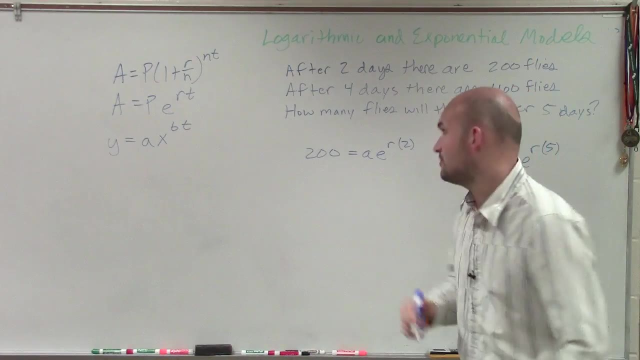 We don't know how many flies initially we started with, nor do we know what the rate is. How are these flies growing right? We don't know that. So let's go back to a little simple equation. if you guys remember, 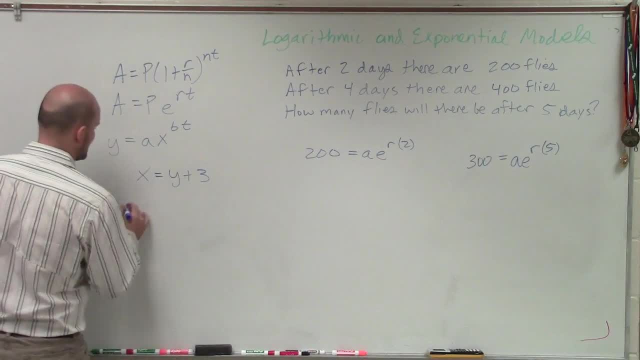 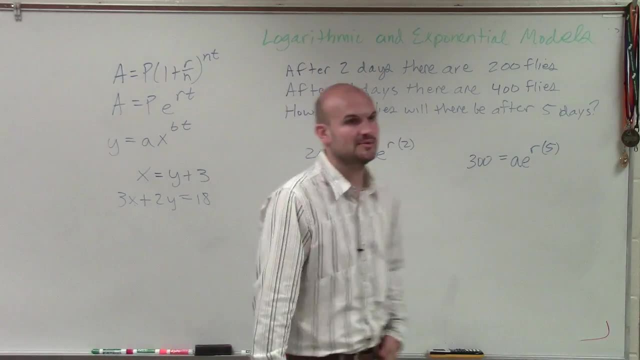 If I had x equals y plus 3, and add another equation: x plus 2y. or let's do: 3x plus 2y equals 18, right, Remember these linear equations. If I had a systems of equations, one of the methods, 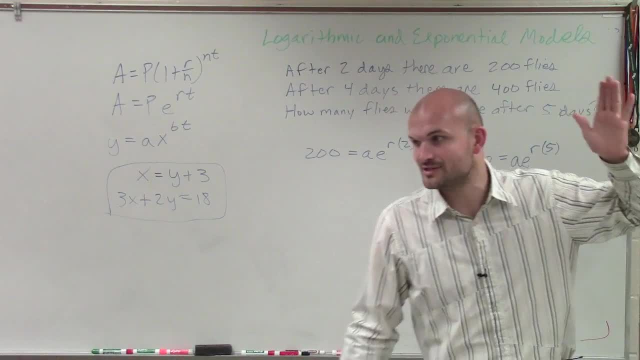 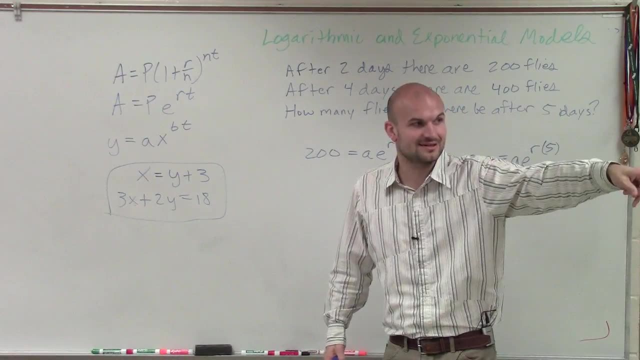 to solve systems of equations. does anybody remember one method that we use to solve systems equations? We could use that, Chris: Solving, Solving, Solving. But how do we solve, though? What's one way to solve? yes, 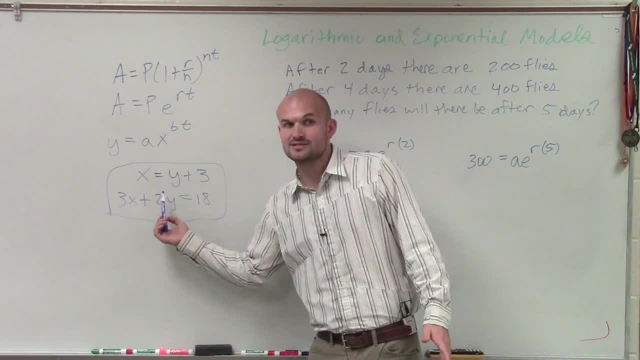 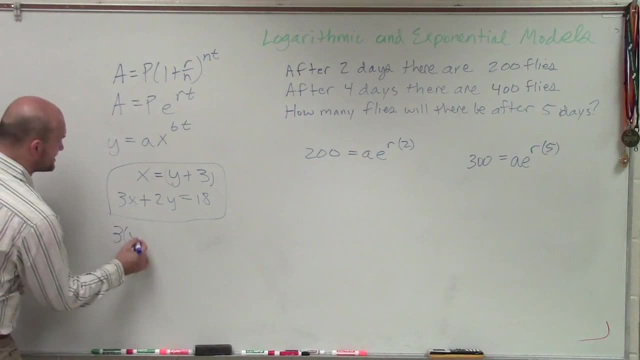 You could apply substitution right Here. we have two missing variables and we have two equations. So one way to solve this was you'd plug in this equation in for x into the other variable. So I'd have 3 times y plus 3 plus 2y equals 18, right. 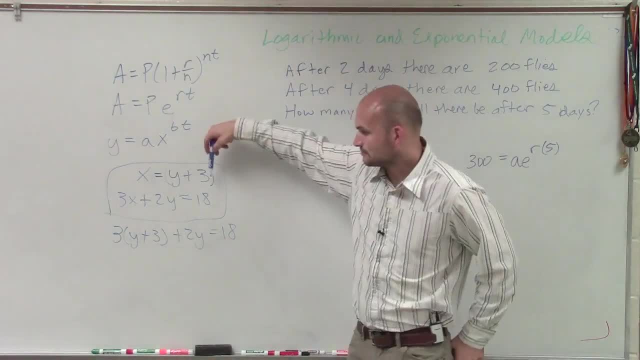 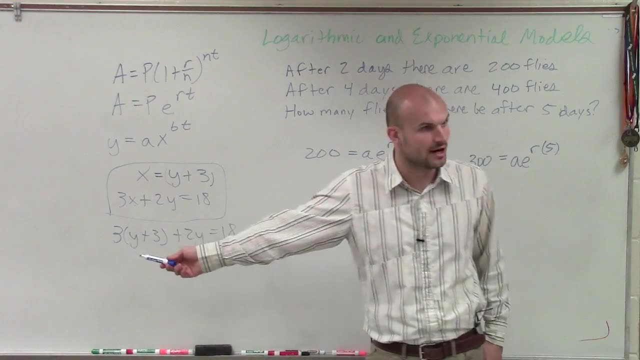 Remember this: algebra 2,, algebra 1, we worked with this. So by doing this then you'd solve for y, And once you figure out what y was, you could plug y back into one of these equations to solve for x, right? 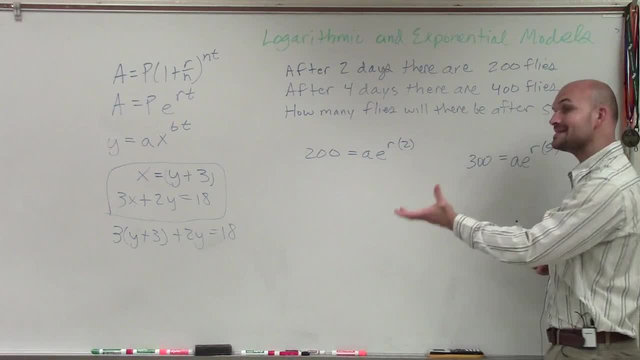 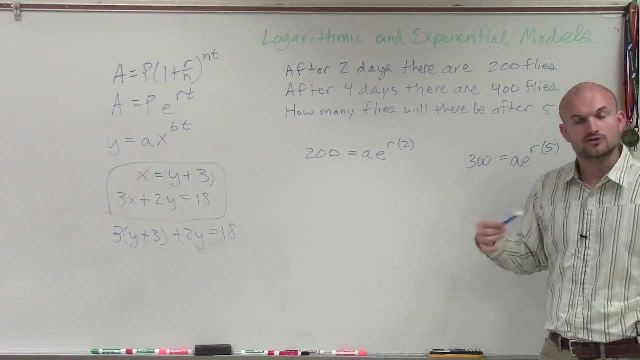 Well, ladies and gentlemen, in here we have that exact same scenario, except they're not linear. We have a is missing and r is missing, But we don't know what a and r are. So what we're going to do is we're 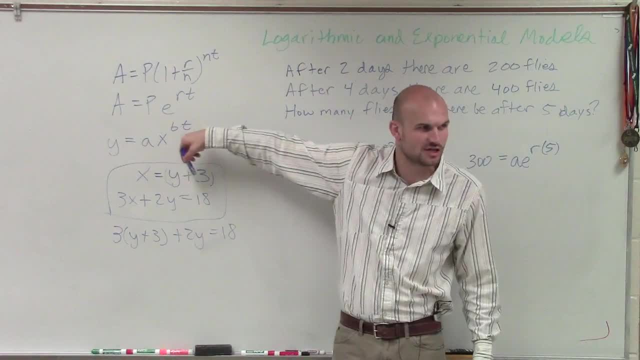 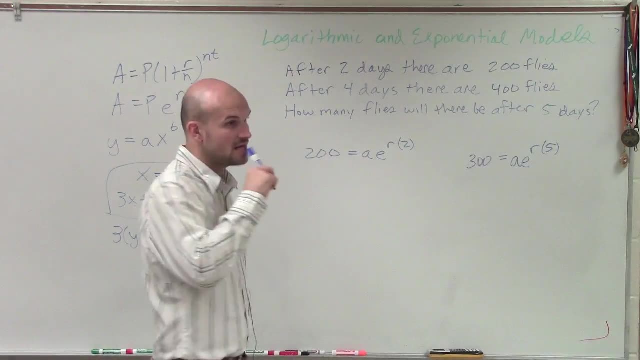 going to solve for one variable. Now, this one was easy to solve for substitution because it was already solved for x. right, Here we don't have anything solved, So what I'm going to do? yes, It's supposed to be 400.. 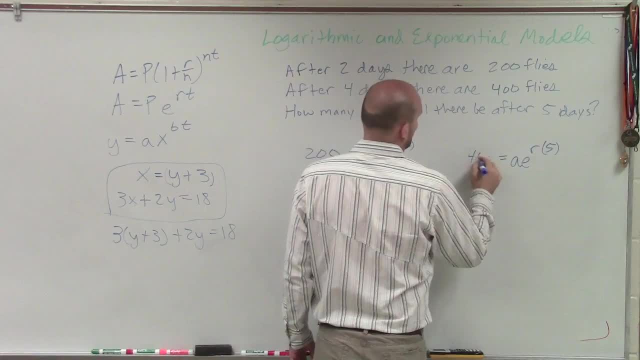 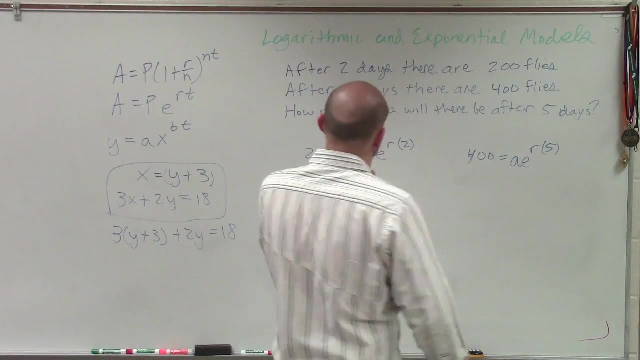 Yes, it is supposed to be 400. So in this case, In this case, we need to solve for a variable If we're going to apply substitution. yes, Wouldn't it be four days? All right, let me just check the problem. 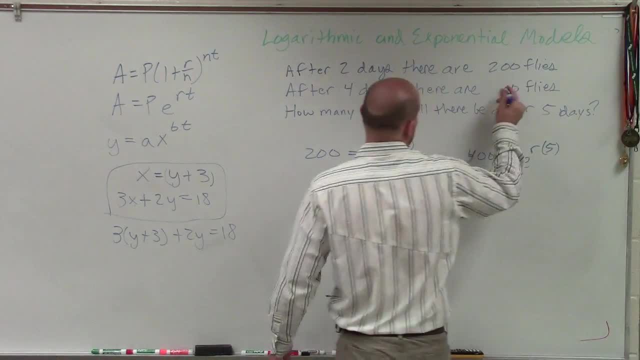 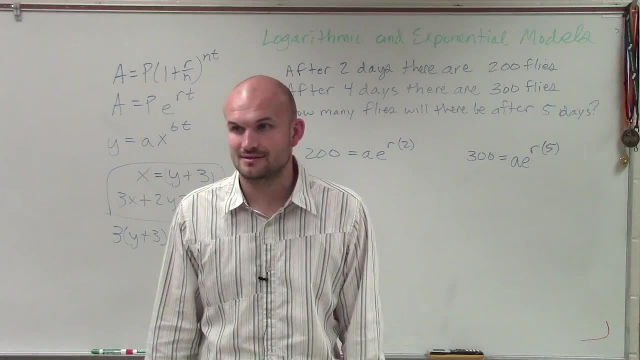 It says after four days there are 300 flies. I just said messing everything up. Oh OK, sorry, After four days there's 300 flies. Yes, So would 10 flies be a total? Yes, thank you. 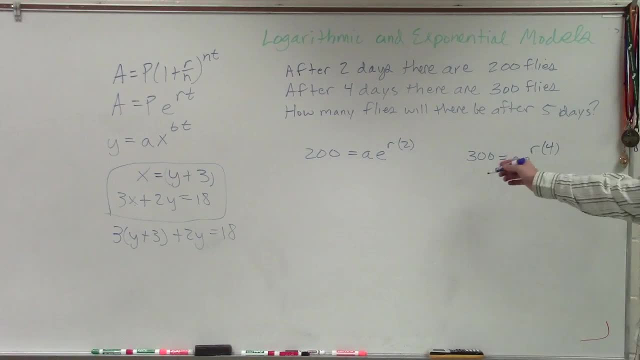 OK, so I wrote down the wrong information. So after four days there's 300 flies, After two days there's 200.. Let's just double check that After two days. oh my, What did I do, Like not write the right problem? 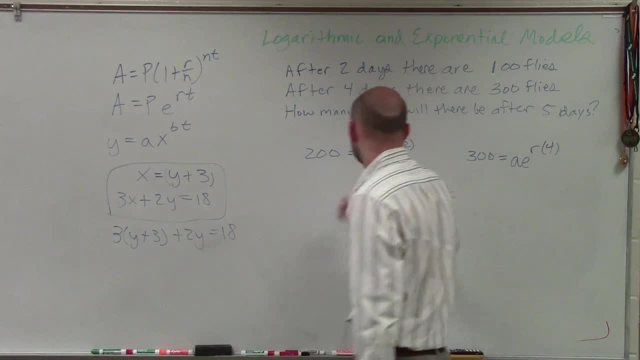 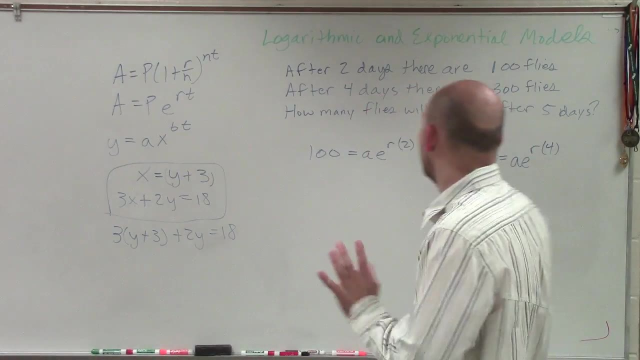 It's: after two days there's 100 flies. Sorry, focus, Geez, oh man, I don't even know where these numbers came from. So after two days we have 100 flies. After four days we have 300 flies. 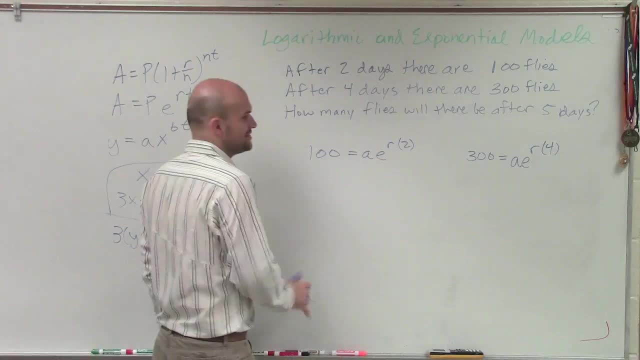 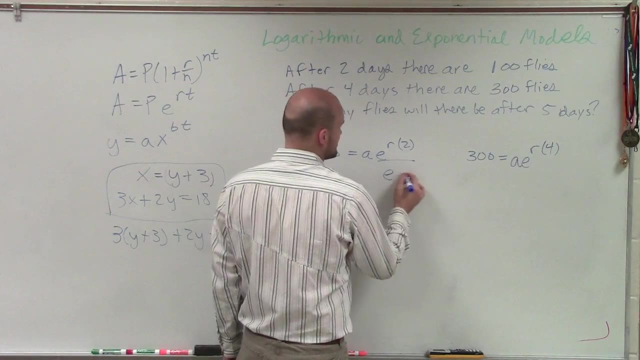 OK, we're good now. So now what I need to do is let's solve for one of our variables. We can either solve for r or a. I think solving for a is going to be pretty simple or easier. It's easier than solving. 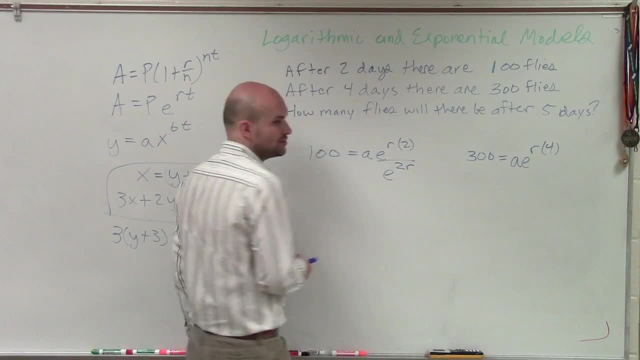 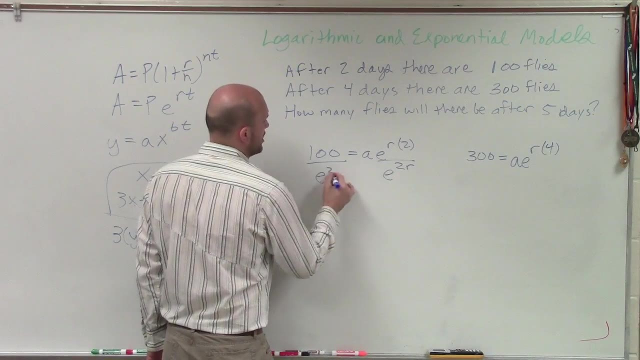 And let's rewrite this: Instead of 2r2, let's just write that it says 2r, right? 3 times 4 is the same as 4 times 3.. So, Chris, do you see that? OK, so then I divide by e to the 2r on this side. 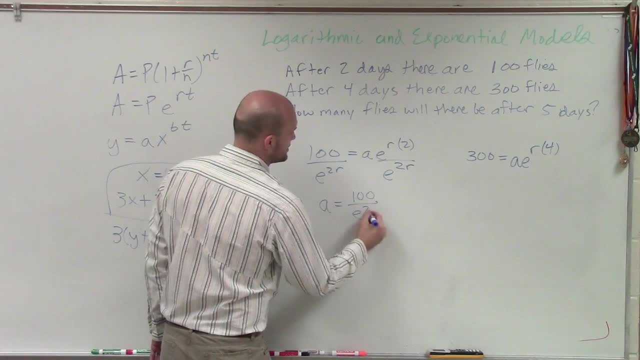 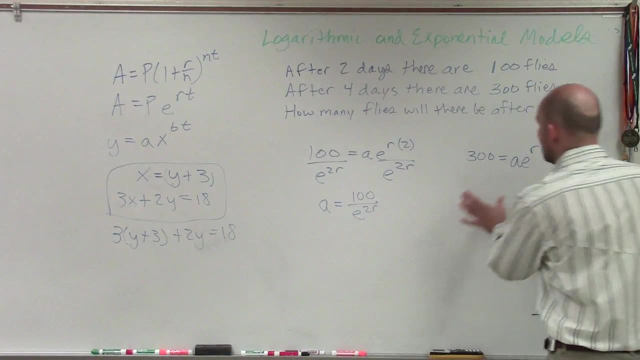 So therefore I can say a equals 100 over e to the 2r. All right, just like we do substitution over here, I'm now going to take what a equals and I'm going to plug it into this equation so we can solve for r. 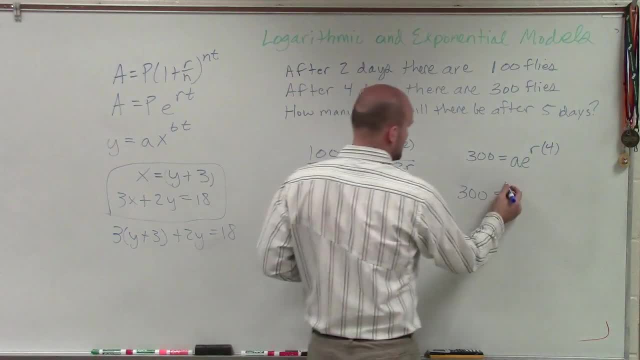 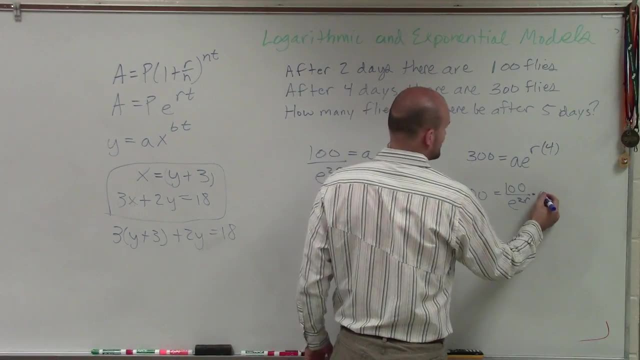 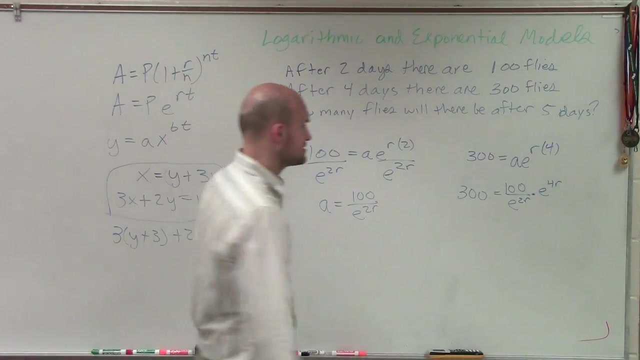 So therefore, 300 equals a, Now equals 100 over e to the 2r, And I'm going to rewrite this as 4r times: e to the 4r. So now I'm multiplying across. So therefore you could say this is really 1.. 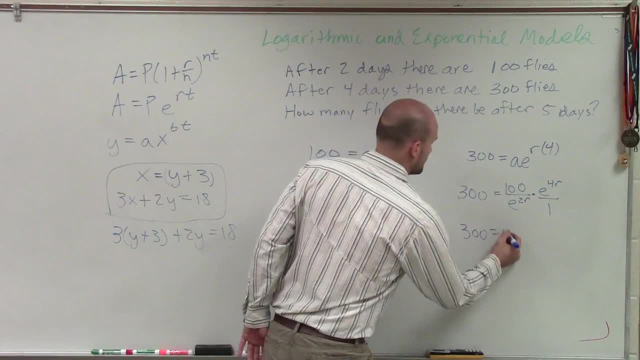 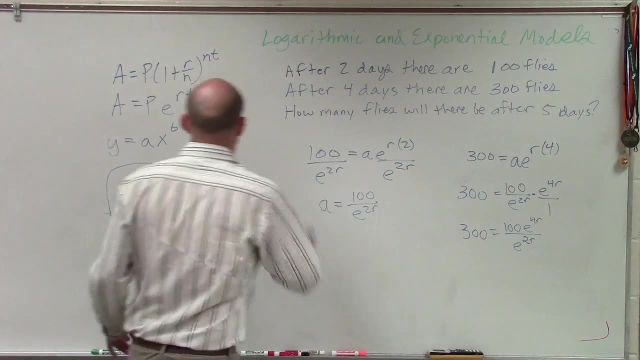 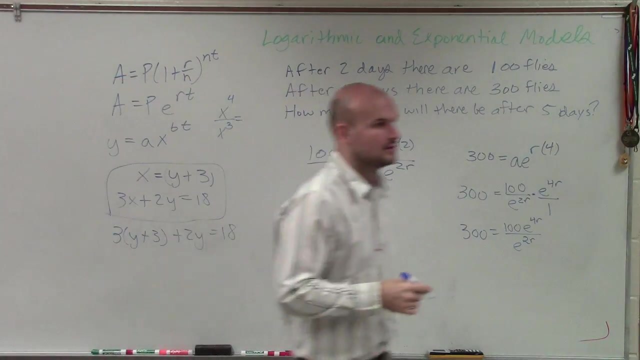 So therefore, I could say: 300 equals 100, e to the 4r divided by e to the 2r. Now, ladies and gentlemen, remember what happens: if I have x to the 4th divided by x cubed, What does that equal? 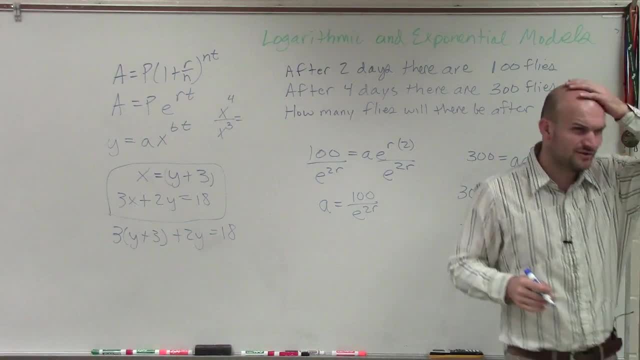 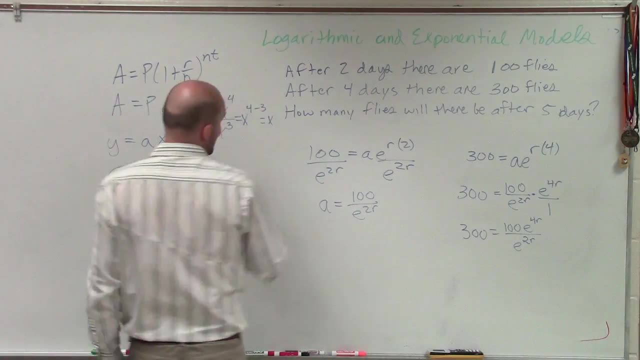 Anybody remember what Jamie did on r? What do you do when you divide? You subtract them right So that equals x to the 4 minus 3, which is equal to x. So over here I have e. Do the e's are the same base right? 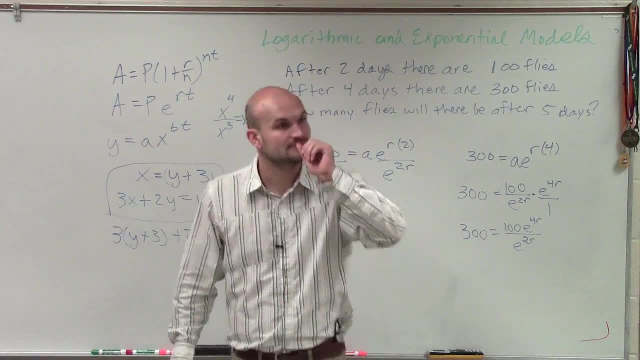 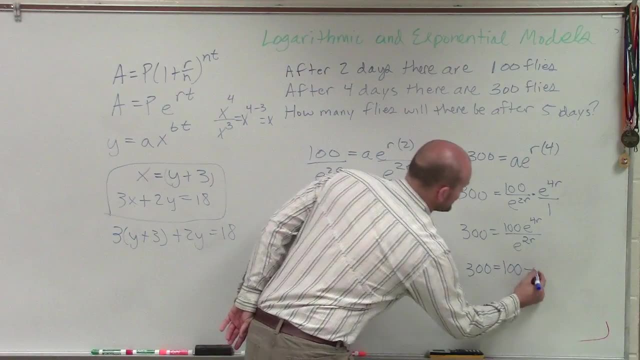 Just like they're variables. But these aren't variables. These represent numbers. Yes, OK, So therefore, to divide these, that's e. So that equals 100 to e. to the 4r minus 2r. Well, 4r minus 2r is just 2r. 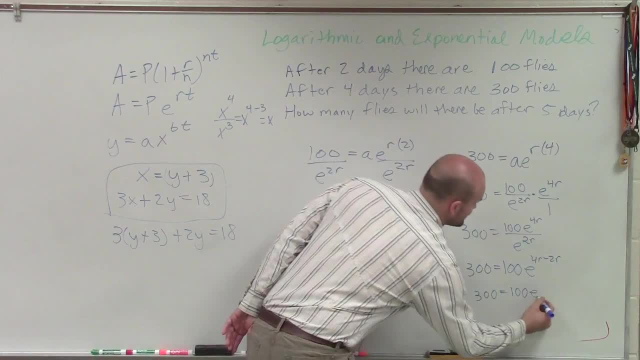 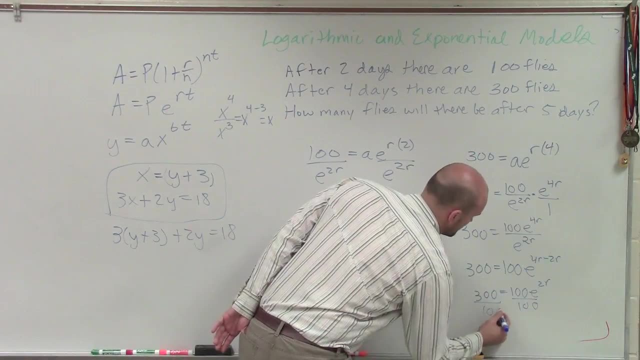 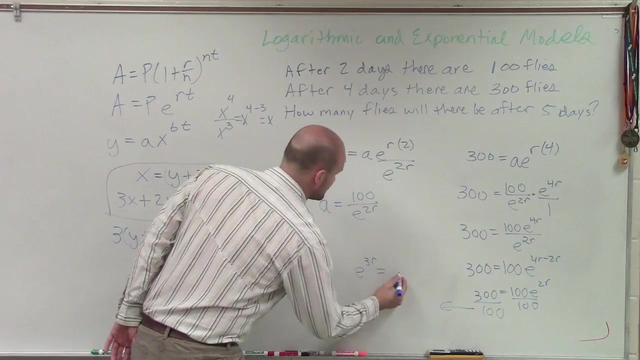 So we could say: 300 is equal to 100 times e to the 2r. Now we still haven't solved for r yet, So I divide by 100. And I'm just going to kind of move this over here. So therefore I have: e to the 3r is equal to 3.. 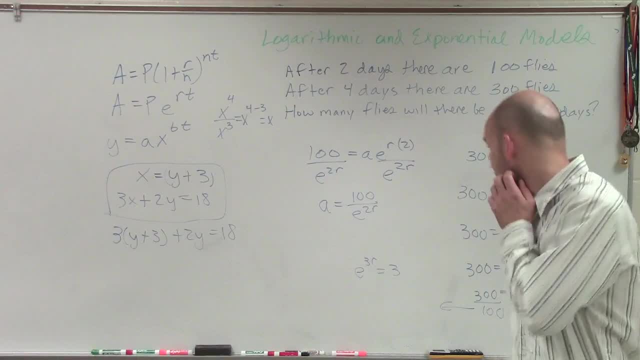 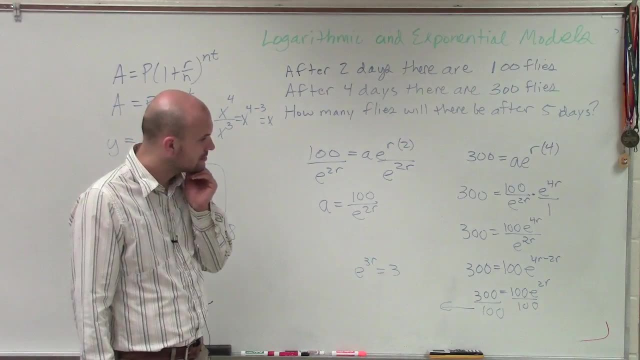 Now going back to your homework: last night we have something. Did I make another 2r, not 3r? We wrote e to the 3r is equal to 3 over the left. Oh yeah, 2r. 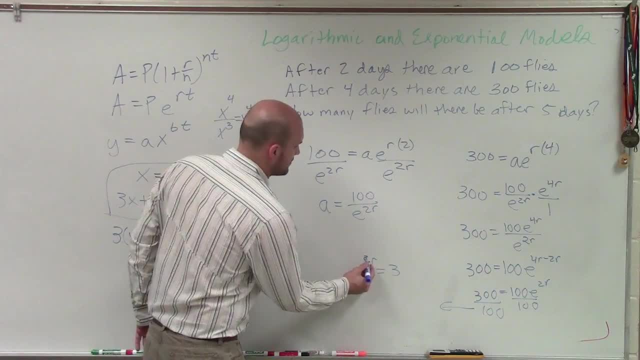 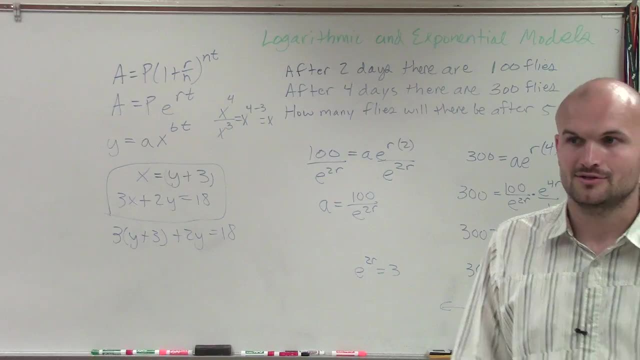 Thank you All right, So right here. So now, going back to your homework from last night. does anybody know what we do in this case, now to go ahead and solve Zoe? do you know what you do next to solve for this? 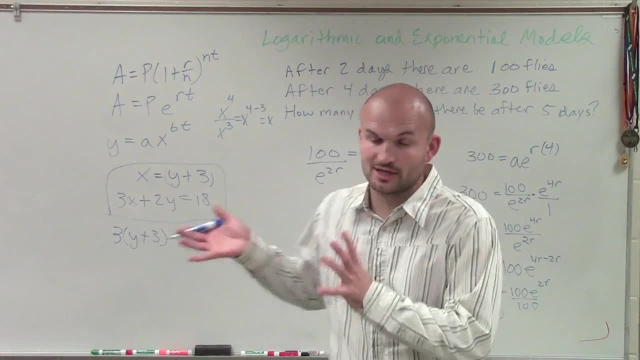 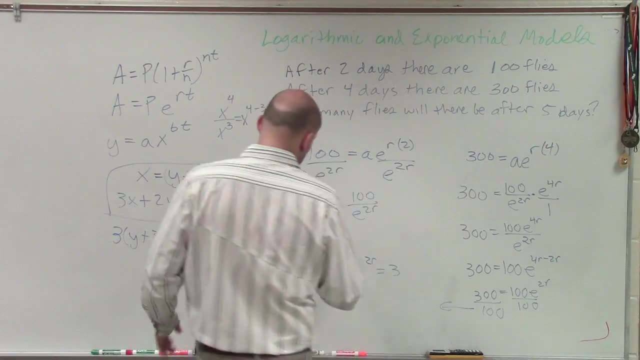 Remember. OK, So remember, we can do this. There's a couple ways We can convert this to exponential form, Or we can take the natural logarithm of both sides. The reason why I like taking the natural logarithm of both sides: 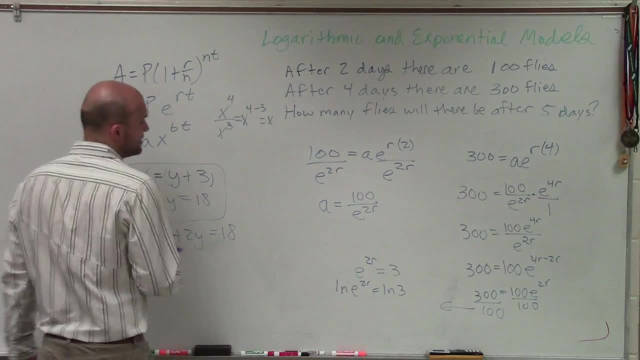 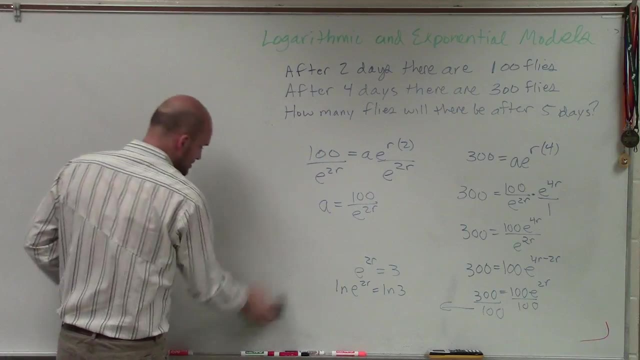 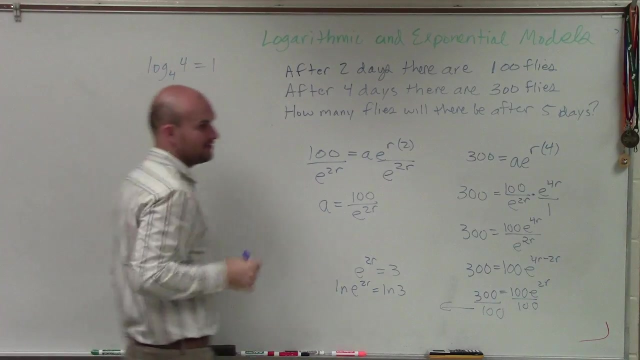 is because by using the properties of logarithms- I know that I'm going to erase this now And all this. So by using the properties of logarithms, if you guys remember, first of all, log base 4 of 4 equals 1, right. 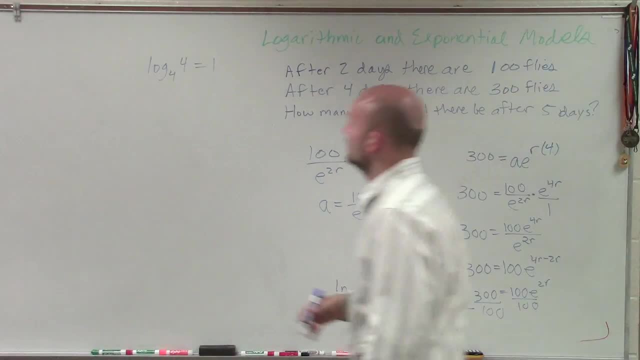 4 raised to what power Gives you 4.. 1, right. And then if I said log base 4 of 4 to the x, that just equals x, Because 4 raised to what power gives you 4 raised to the x. 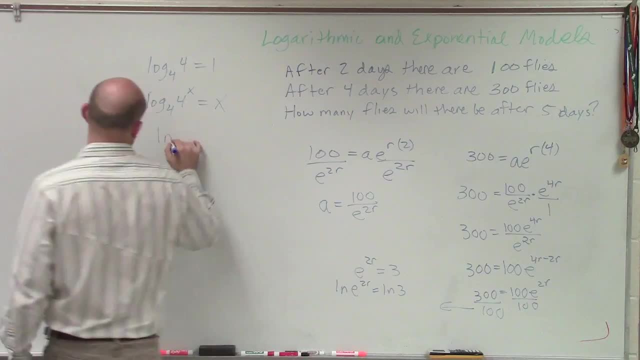 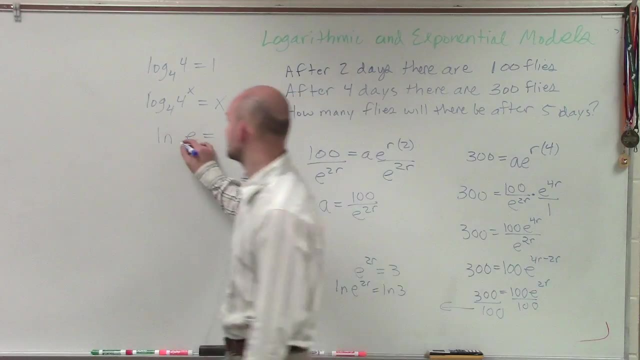 Well, that answer obviously just has to be x. Well, ladies and gentlemen, that works the exact same thing with natural logarithms Because, remember, a natural logarithm has a base e, which we don't write in there all the time. 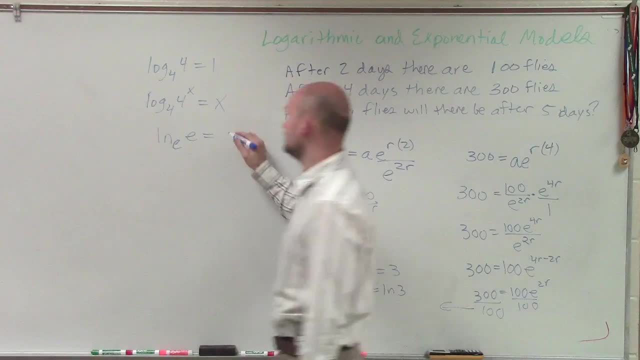 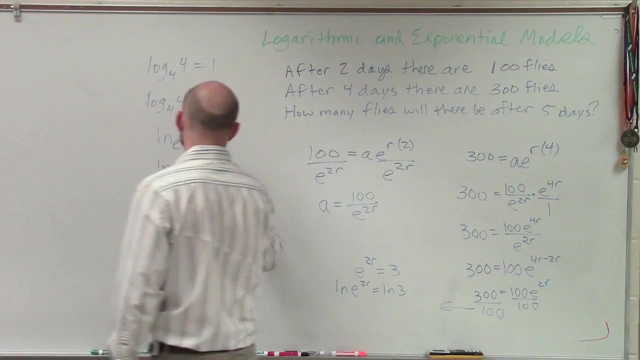 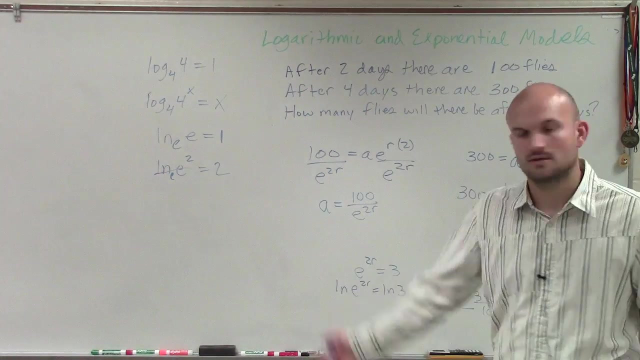 So you can write in the base e e raised to what power gives you e? First, If I said ln e e to the second power or ln of e to the second power, that's just going to equal 2.. Because the ln base e of e, we know it just goes to 1.. 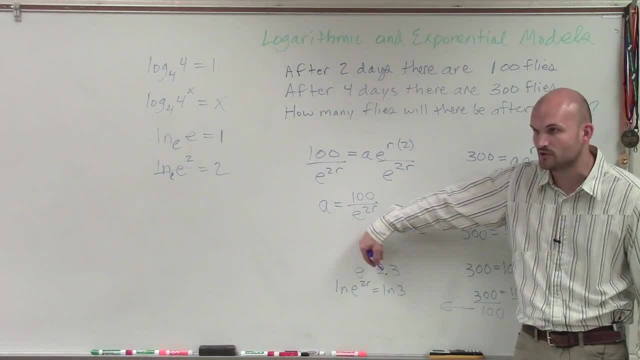 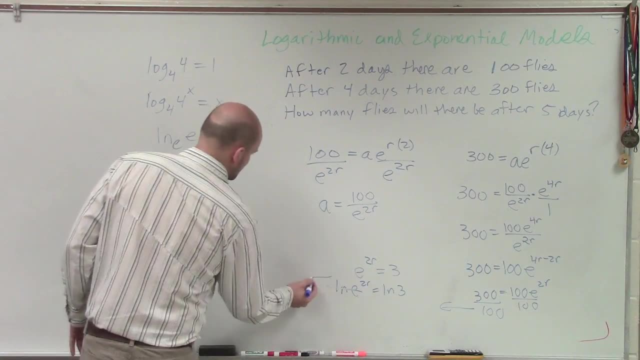 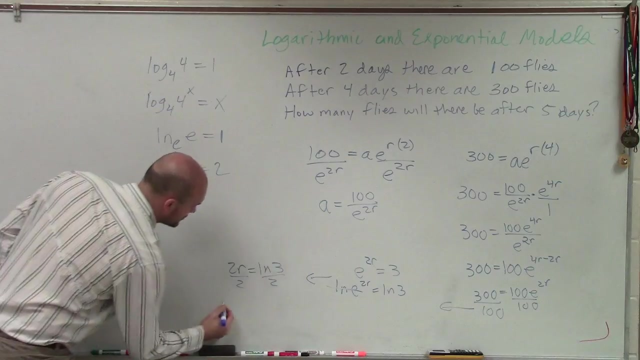 So, therefore, it equals 2.. So, ladies and gentlemen, when I take the ln of both sides, now, this ln goes down. So now I'm just left with 2r. equals ln of 3.. Divide by 2.. Divide by 2.. 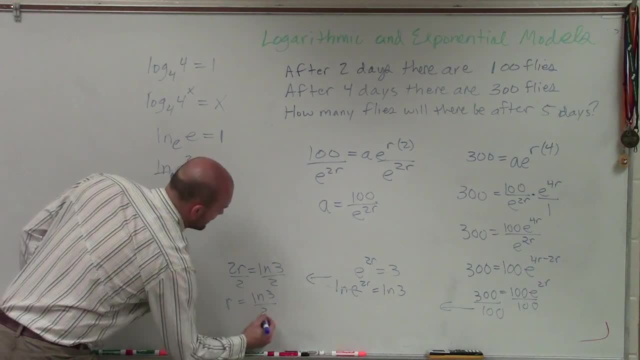 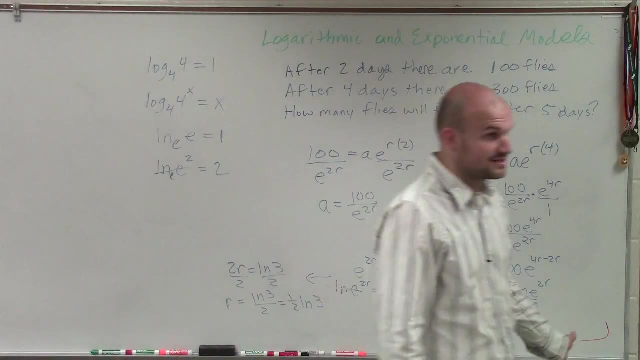 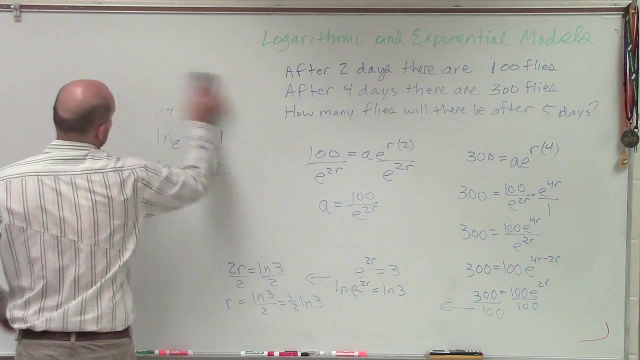 r equals ln of 3 divided by 2.. Or we could rewrite that as 1 half ln of 3.. So now, ladies and gentlemen, we know what r is, r rate, which I'm going to leave right now as 1 half ln of 3.. 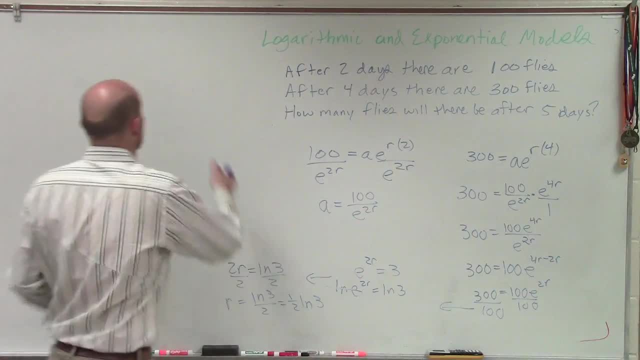 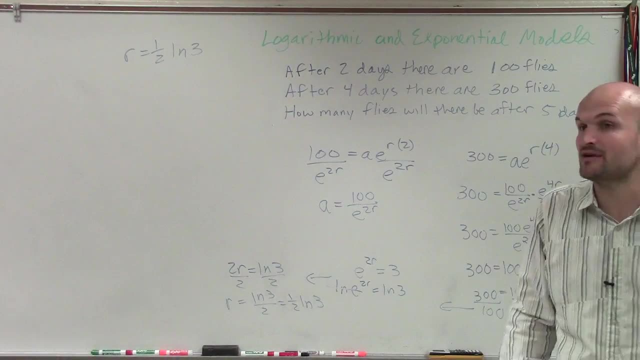 So we figured out what the rate is. These flies. they grow at a rate of 1 half ln of 3.. Now that's not what the question is asking us. The question is asking us: how many flies are they going to be? 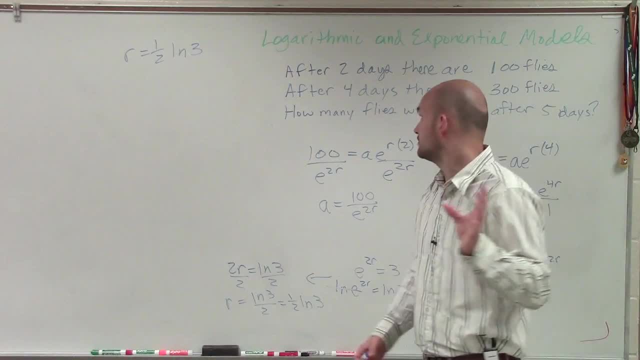 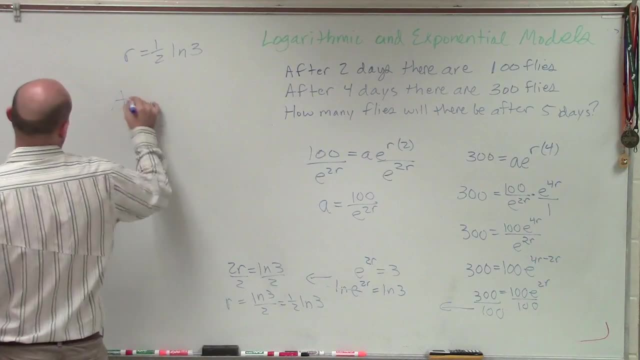 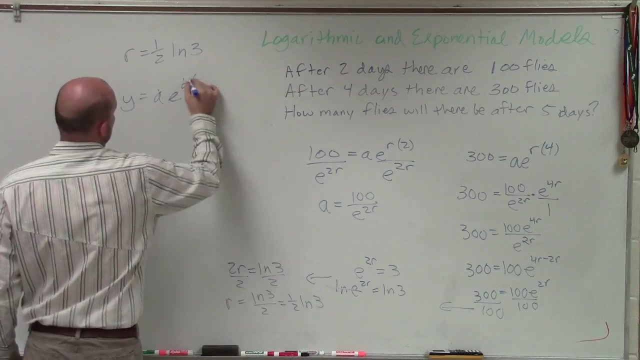 How many flies are they going to be after five years? I'm sorry, after five days. So now, what we need to do is we need to start with. well, what do we start with? Remember that a or y, y equals a times e to the bt. 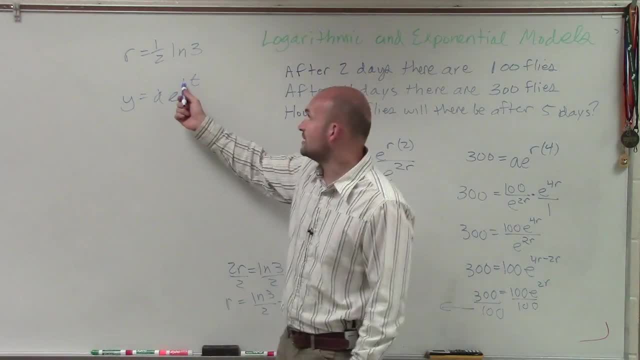 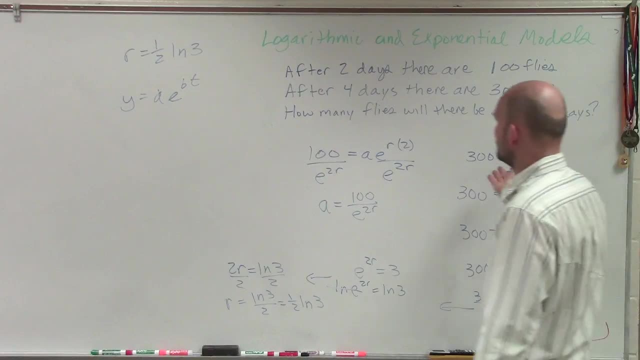 We need to figure out what a is our initial amount. We know what r is, or our b. Why did I start writing it as? Oh, I started using r. OK, Oh right, this is r. r represents your rate. 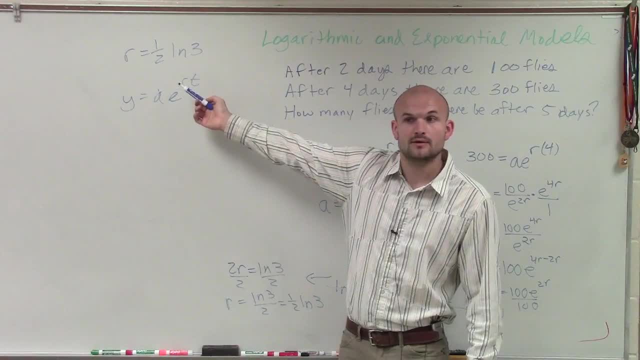 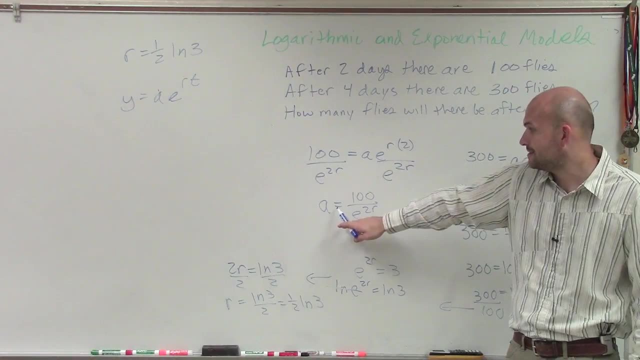 So we have this as our r right. We know what r is now, But our problem is now: we don't know what our initial amount is. Well, remember, our initial amount is a. So now, what I can do is I can plug in what r is. 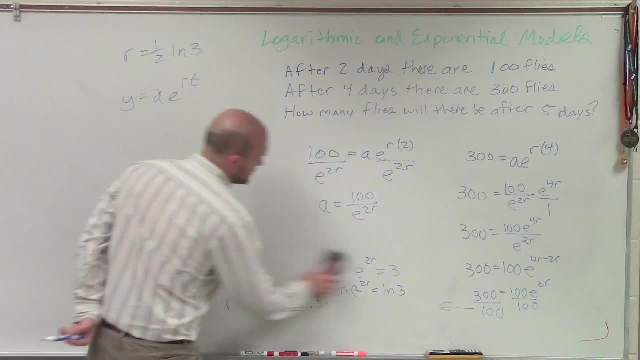 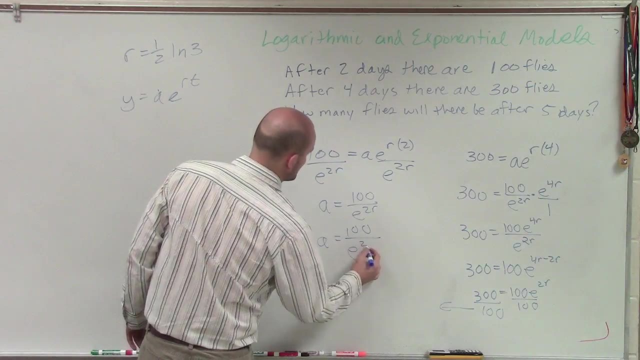 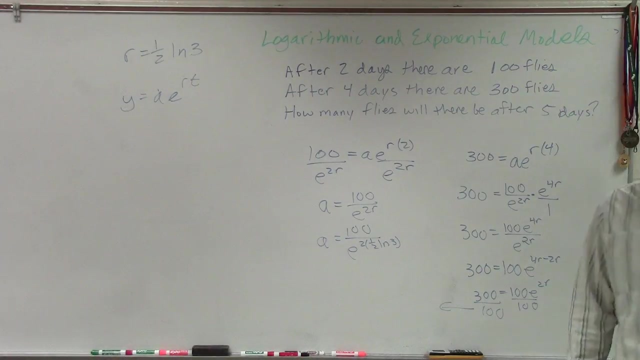 into this equation. So I have: r equals 1 half ln of 3.. So now, when I plug this in a, equals 100 divided by e to the 2 times 1 half ln of 3.. All right, Now, property of logarithms. when we use our one-to-one. 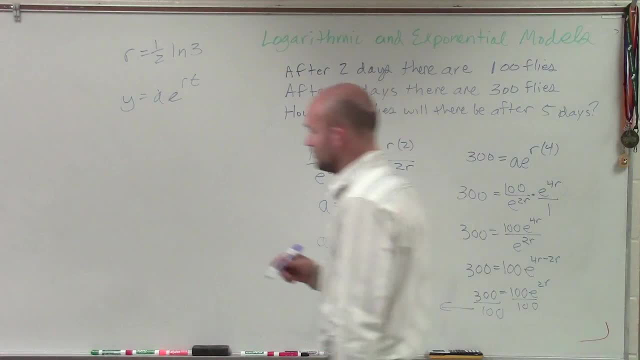 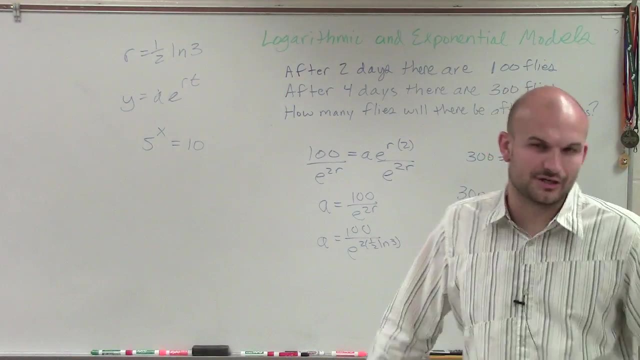 properties. there's a couple things that I want you guys to go over. If I have 5 to the x equals 10, using my one-to-one properties, Julianna, do you know what I would do to solve for this If I said 5 raised to the x equals 10,? 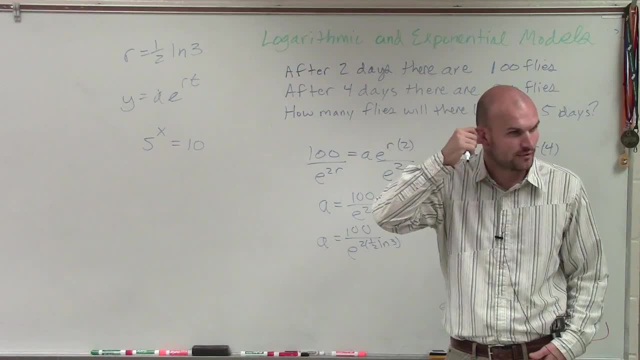 I could take the log of both sides. That's one way. And what base of log would I use? 5. 5, right, Exactly because when you take log base 5, you get a log base of 5.. 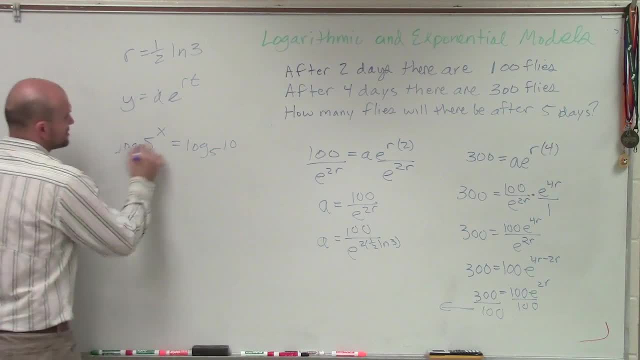 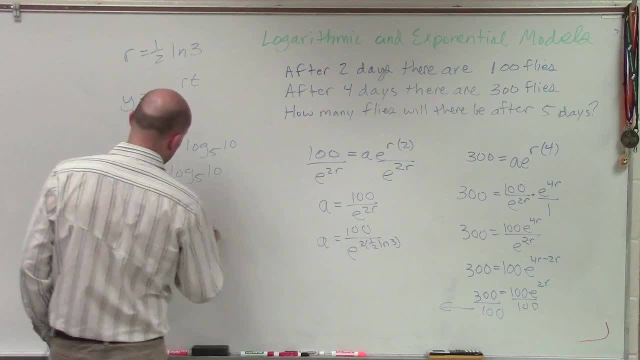 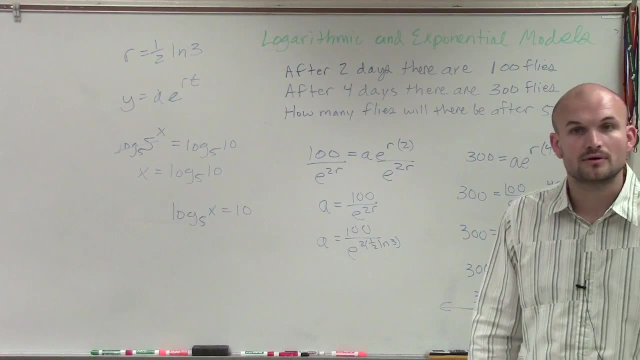 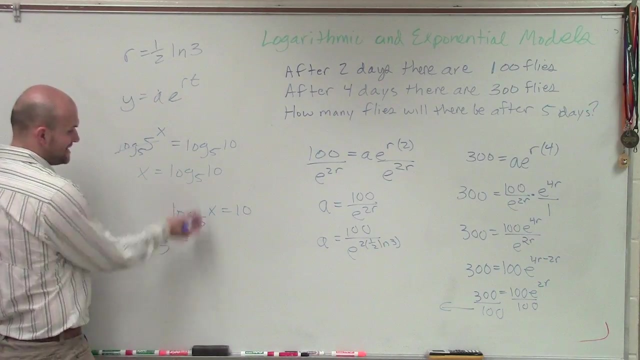 OK, Now what about if I already said log, base 5 of x equals 10?, And I wanted to solve for this. Another way what you can do, Ahmad, is you can now raise this to the fifth power Or, I'm sorry, keep this, raise these with a base 5.. 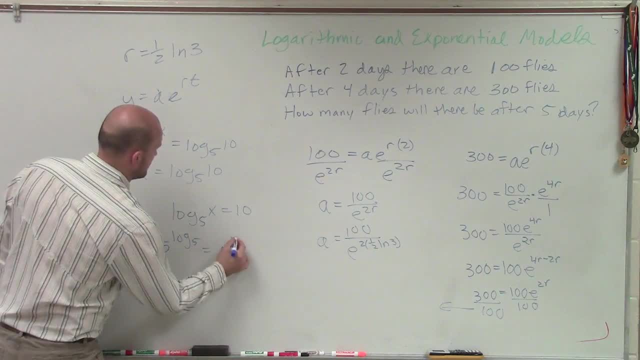 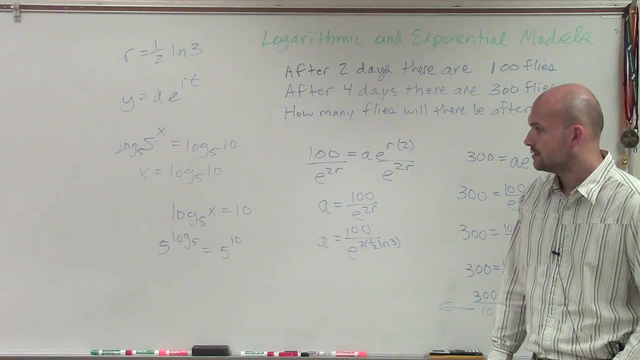 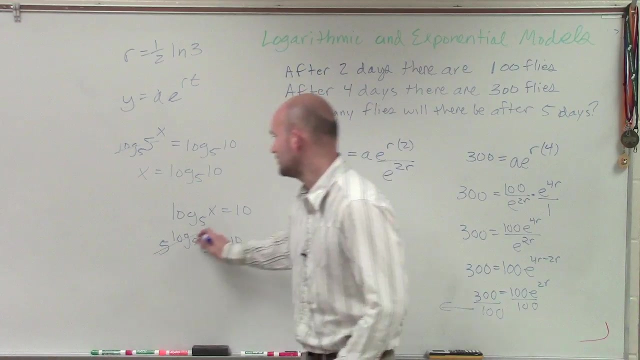 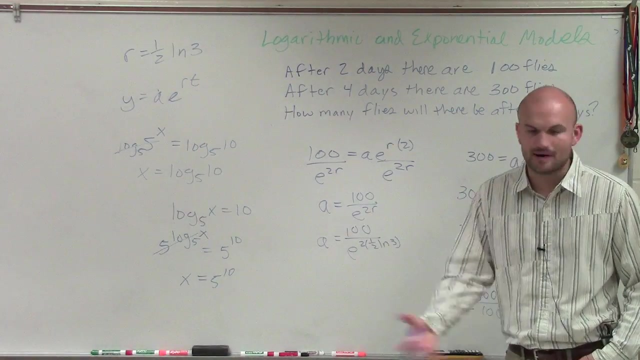 That is another one of our properties. Therefore, that's to the x. So therefore, if you take this and you raise these to the power, that again just goes to x. All right, that's one of our properties again. 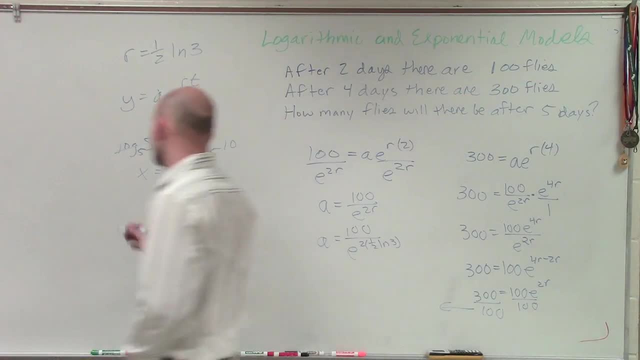 for logarithms which state: if you have, let me go and write it to you. If I talk to you guys about this log base, 5 of 5 just equals 1, right? Well, 5 raised to the log base 5, that just equals 1 as well. 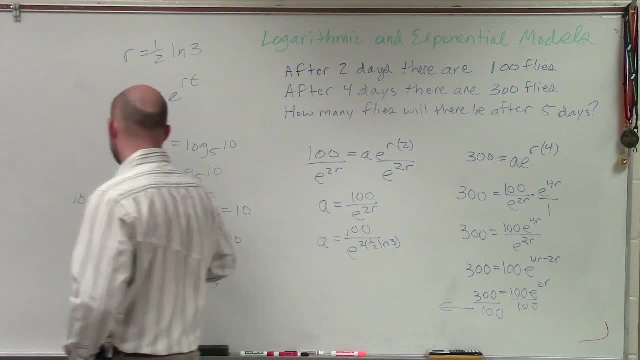 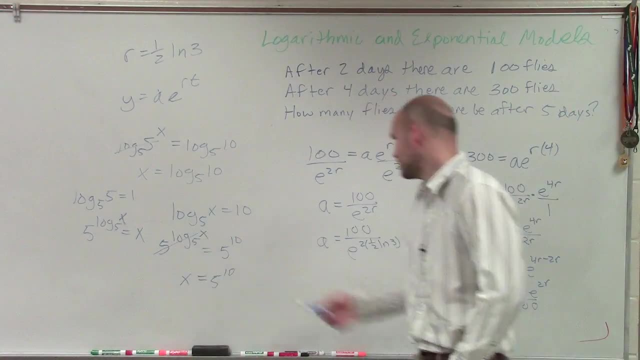 Let's see if I have this equal to x. If you take 5 and you raise it to the log base, 5 of x, that's going to equal x. So what I want you guys to understand is: those can go out. The reason why that comes into play here: 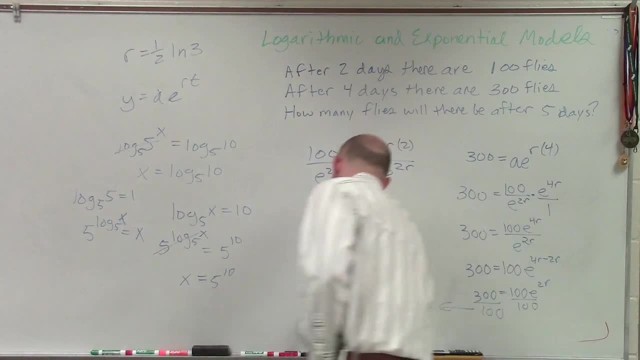 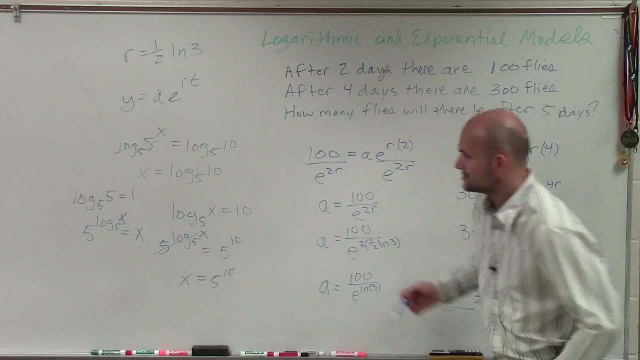 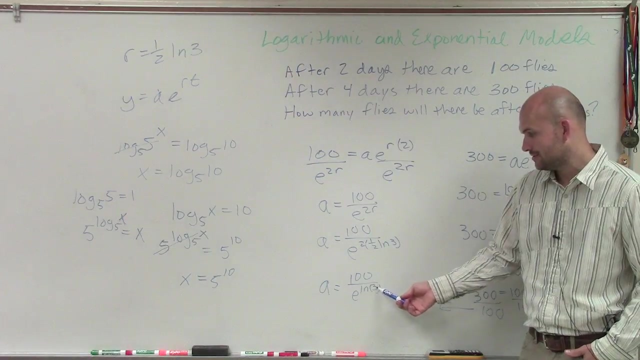 is because now 2 times 1 half, that's just 1.. So I have a equal to 100 over e to the ln of 3.. Well, just like I have 5 raised to the log base of 5,, if I have e raised to the ln, that's just going to equal 3.. 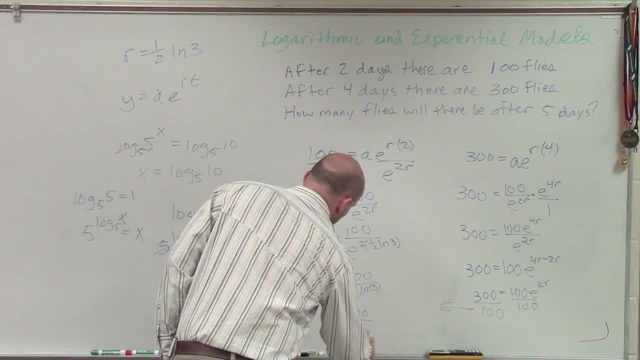 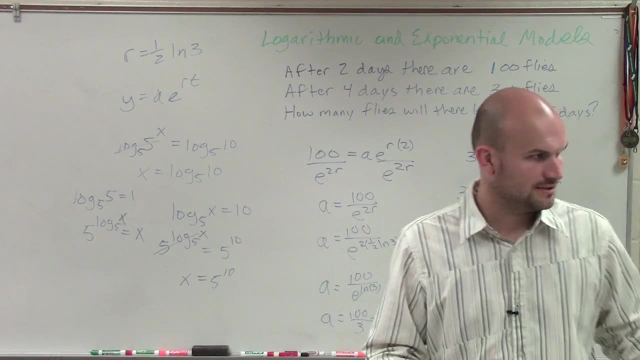 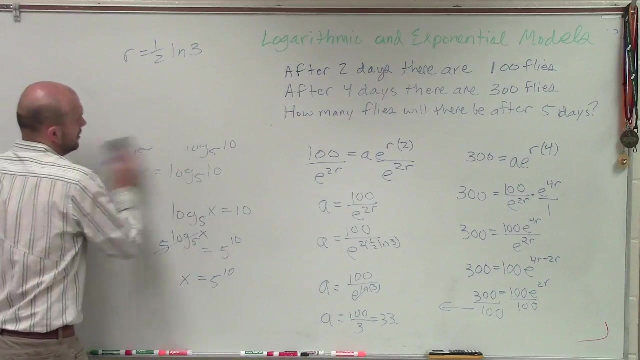 So therefore, a equals 100 over 3,, which equals 33.33333.3.. But obviously we know we can't have a third of a fly, right, Yeah, can't have a third of a fly. So we're going to say our a is just going to equal 33.. 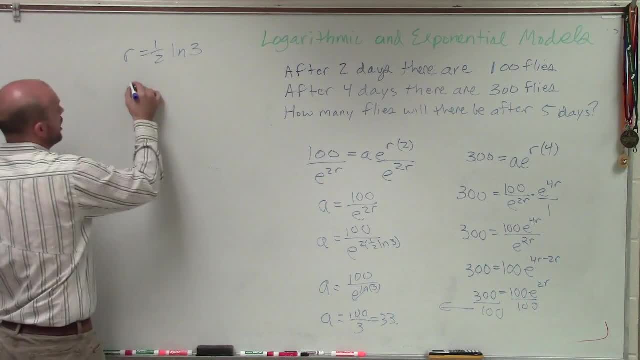 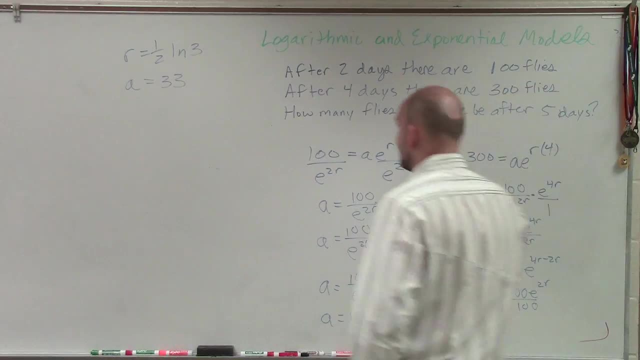 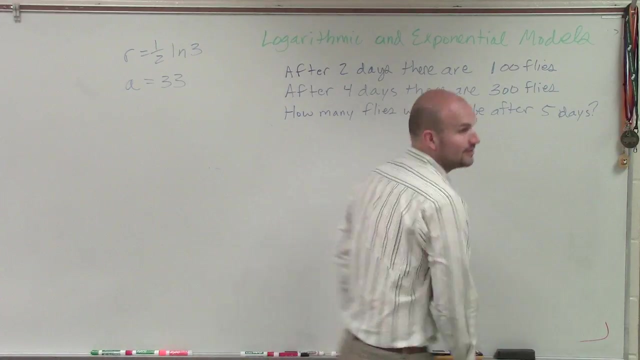 OK, so now we've found our r and we know our a equals 33.. So now what we need to do is now find this amount at five days. Yes, please ask questions. Oh, OK, it's OK, I'll go ahead and try to read back and explain. 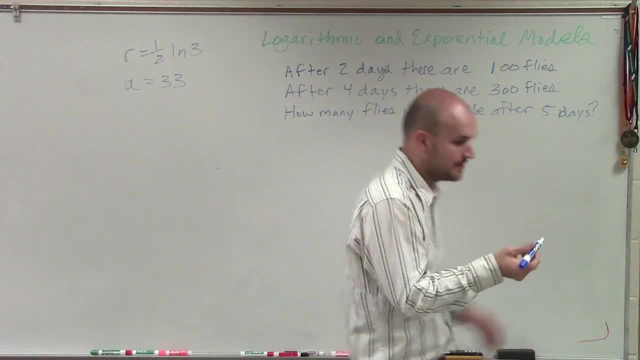 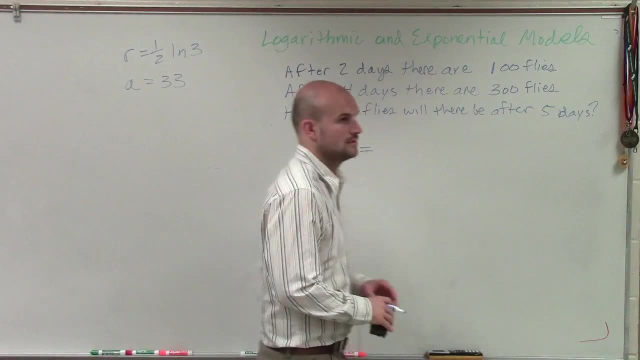 Question: When a equals 100 to e to the 2 and 1 half ln of 3, how did you get e to the ln of 3? on the bottom Is 1 half, e to the 1 half. 2 times 1 half is 1.. 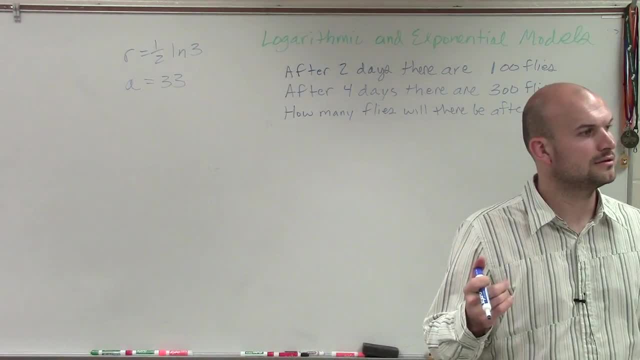 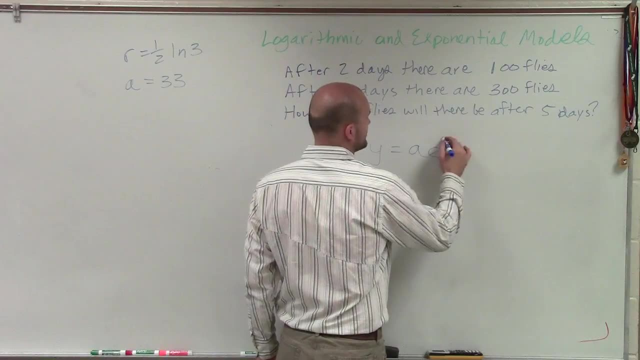 So it just turned to ln of 3. See the 2 times 1. half. that just went to ln of 3. So let's go back. So y equals a times e to the rt. I used bt originally, but it could be r. 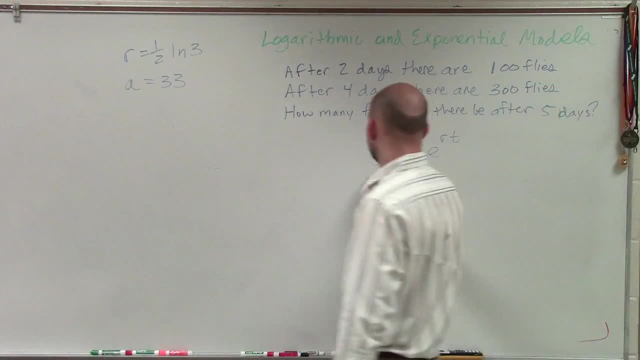 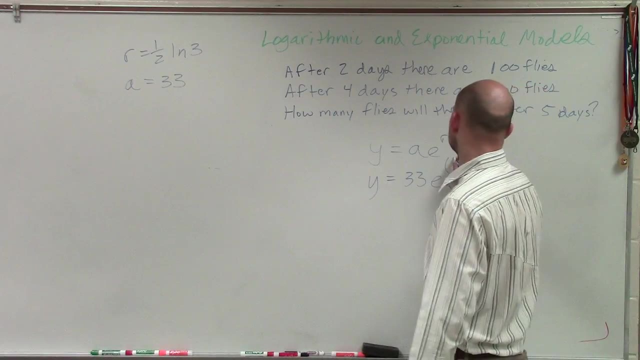 r represents rate. So now we want to figure out what is the final amount after five years. We know that a is 33.. e is going to be our constant. We have our rate, which is 1 half ln of 3 times our t. 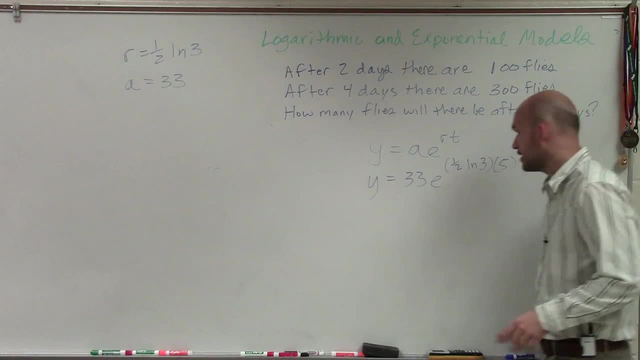 which is five days. So now that we've figured out our a and our t, now we just need to plug this into our calculator. So I'll do 0.5 times ln of 3 times 5.. And then I say: take e, raised to the second answer. 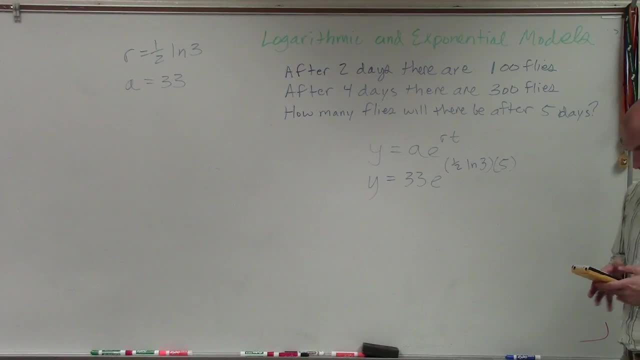 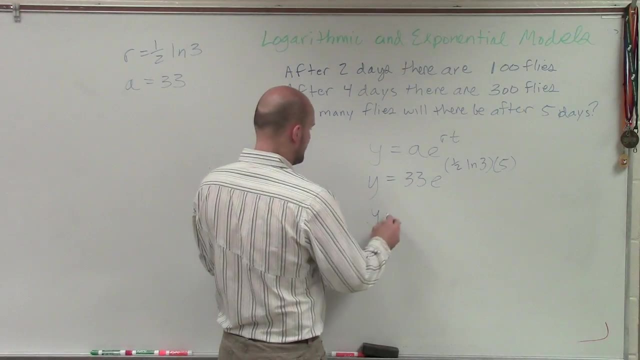 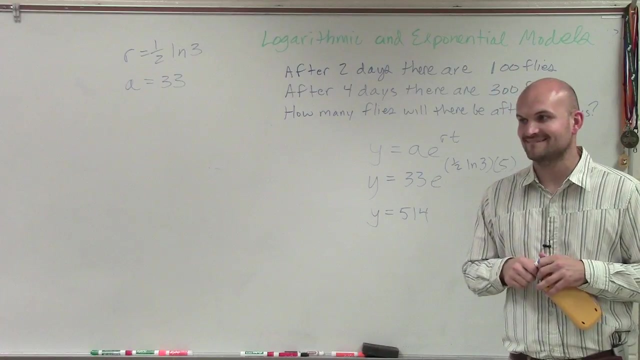 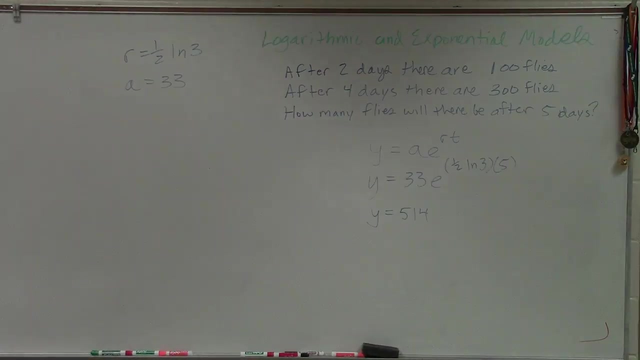 And then I multiply that by 33, and I get 514.41.. Well, obviously, ladies and gentlemen, you can't have 0.41 of a fly. So our final answer is: 514 flies. OK, Yeah, Yeah. That's why you guys have six problems tonight. 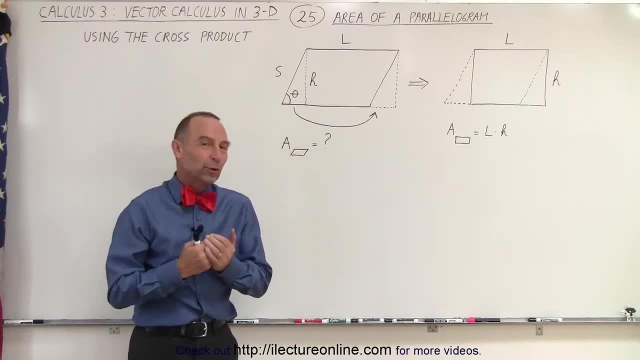 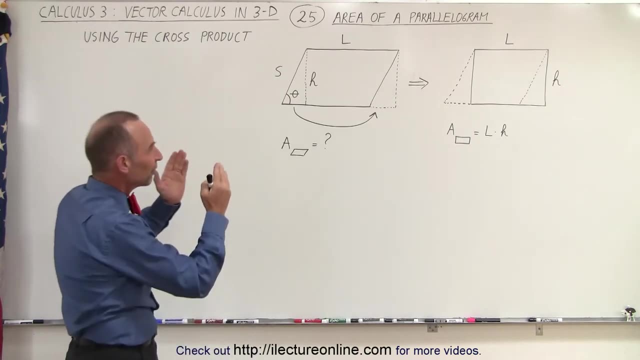 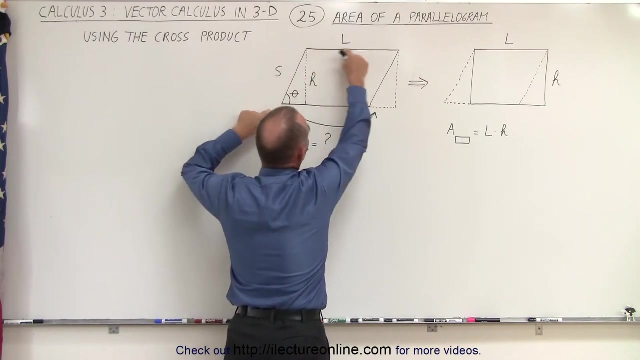 Welcome to iLecture Online. In this video we're going to show you how to find the area of a parallelogram using the cross product, But first let's get a visual sense of what's going on here. So here, with the solid black lines, we've drawn a parallelogram The length of the top and bottom. 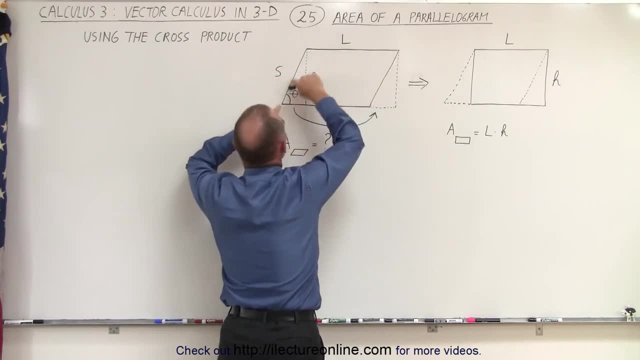 edge of the parallelogram. let's call that equal to L, and this is the length of the side of the parallelogram. let's call it S, And that would of course be S on both sides, so we can write one. 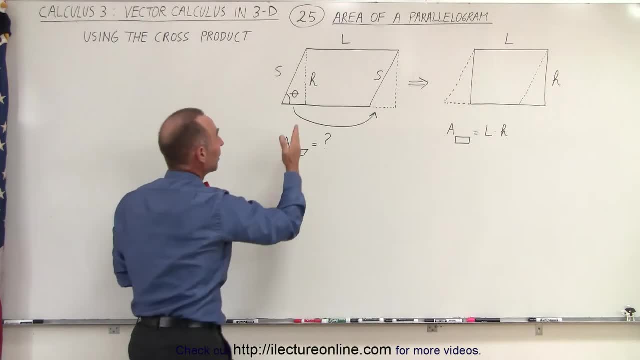 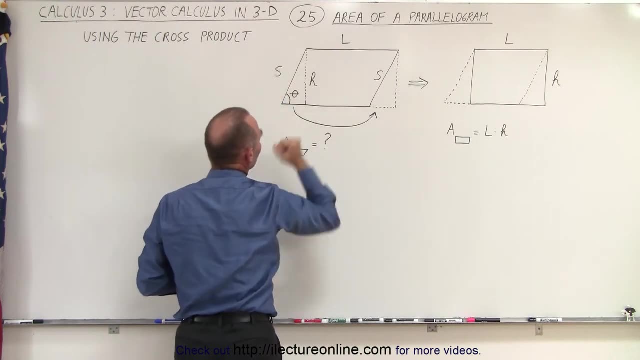 there as well, And then the height of the parallelogram can be defined by this dashed line right here. And then we have an angle between the side on the left side and the bottom side right there. we'll call that theta. Now notice that if we were to cut this little piece off and take that 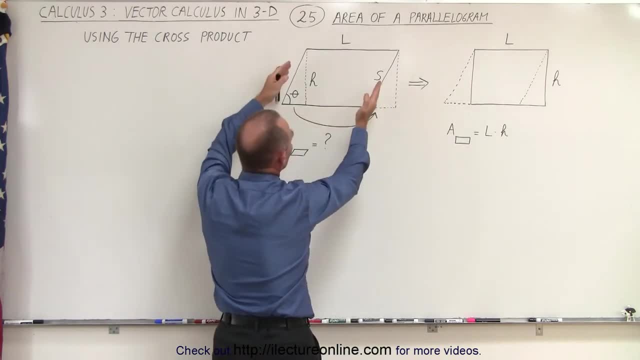 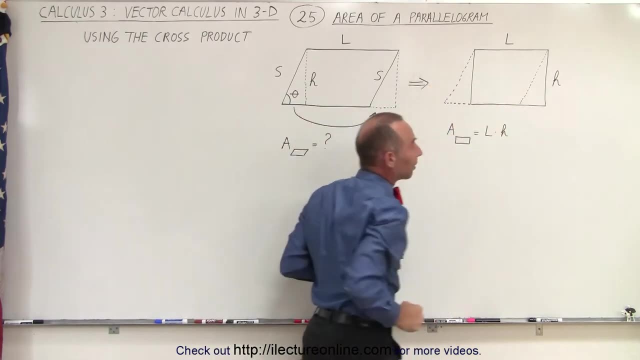 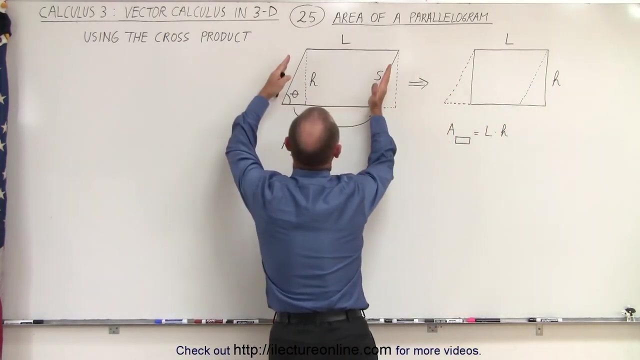 little piece and move it over here. we would then turn the parallelogram into a rectangle which we've drawn right here with the solid lines. The dashed lines represent the original parallelogram. so you can see here that the area of this rectangle would therefore be equal to the area of this parallelogram. Now the 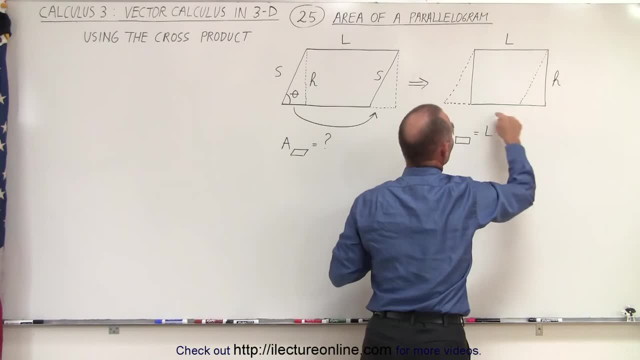 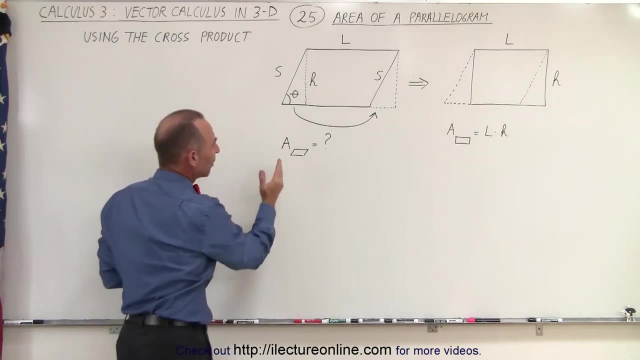 area of the rectangle will be equal to the length times the width. in this case, we have L times H, H representing the width of that rectangle. So the question now is: how do we find the area of the parallelogram? Well, that means we need to find the value for H and, taking a look at this triangle, 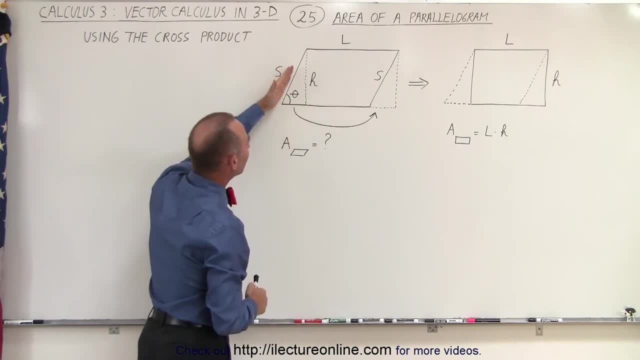 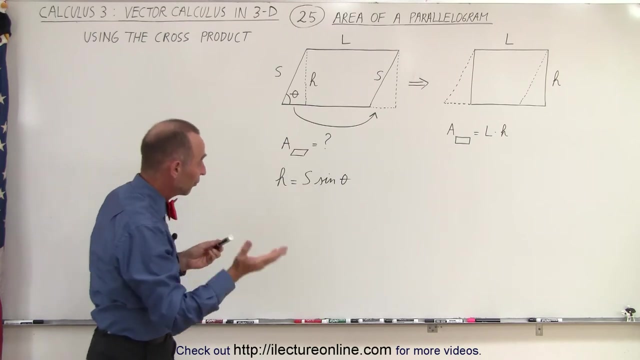 right here we can see that H is equal to the hypotenuse, which is S times the sine of the angle theta. So let's write that down, so we can see that H is equal to the side, S times the sine of theta. Now the next thing we're going to do is: well, first of all, you can